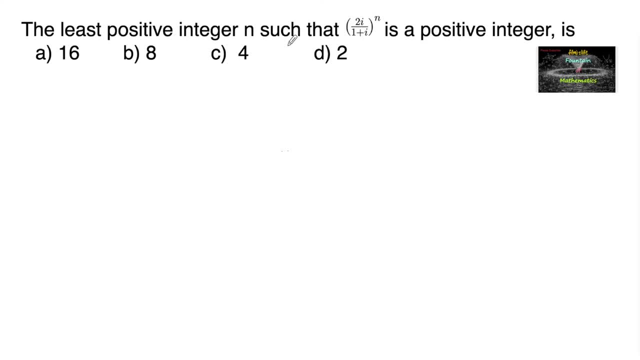 The least positive integer, n, such that 2i upon 1 plus i, whole to the power of n, is a positive integer. So let us consider 2i upon 1 plus i, which equals to 2i, into 1 upon 1 plus i. 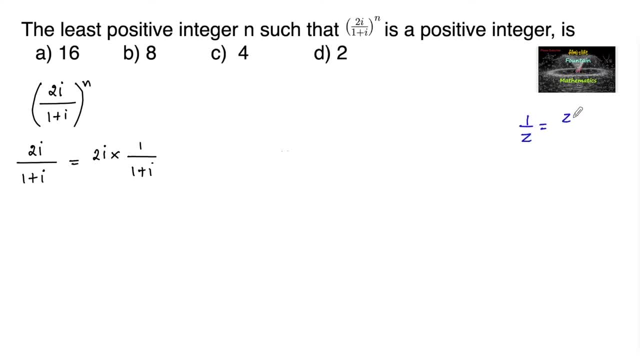 And since we know that 1 upon z is equal to z bar upon mod z whole square, So if z is equal to 1 plus i, z bar is equal to 1 minus i- it's conjugate- and mod z is equal to root over 1 plus. 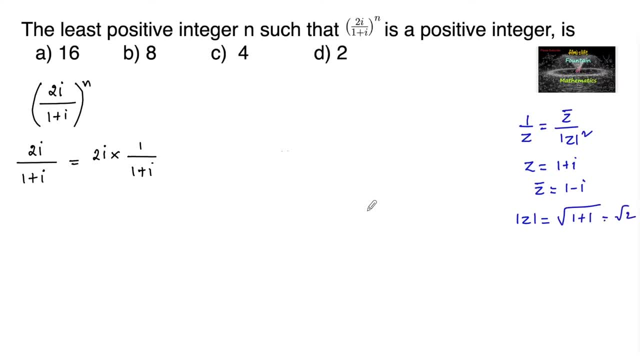 1, which is equal to root 2.. So mod z square, we can write root 2, whole square is 2.. So we can write this is 2i into 1 minus i upon mod z, whole square is 2.. So which is equal to i times of 1 minus i, which is equal to i minus i square, which is equal to i. 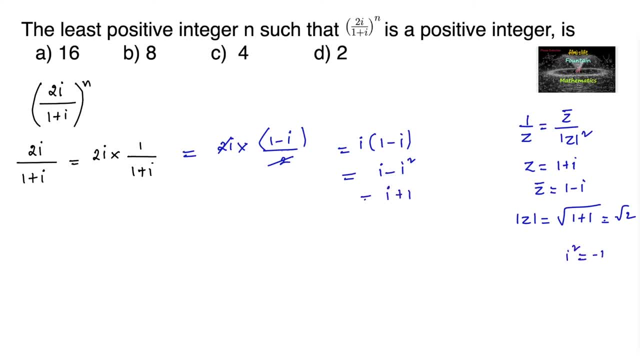 plus 1.. Since i square is equal to minus 1.. So we got 2i upon 1 plus i is equal to i plus 1, and we required a least positive integer n, such that 2i upon 1 plus i whole to the power of n must be a positive. 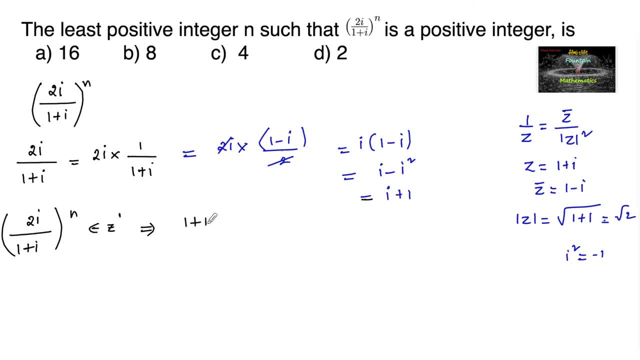 integer. So that is why 1 plus i whole to the power of n must be a positive integer. So let us select from the options. n is equal to 2.. So we have 1 plus i whole to the power of 2, which is equal to. 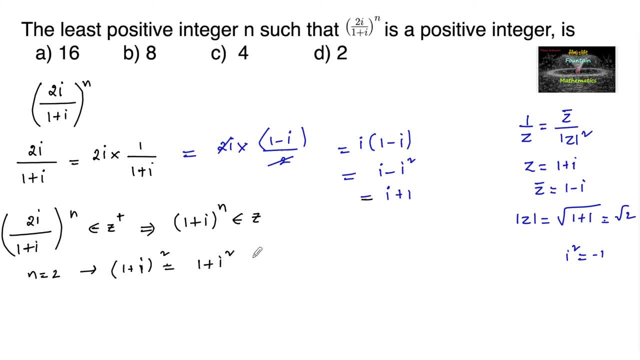 1 plus i. square plus 2i, which is equal to 1 minus 1 plus 2i is equal to 2i, which is not an integer, It's an imaginary number. And now let us consider: n is equal to 4.. 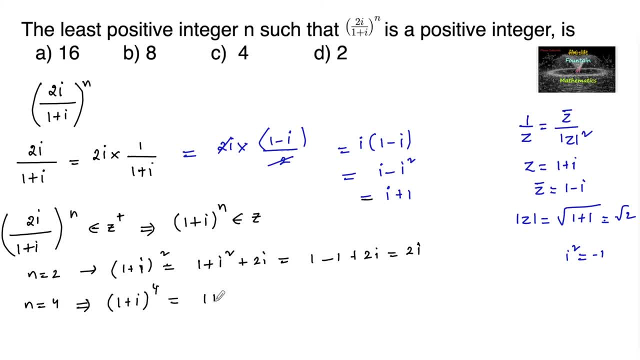 That is 1 plus i whole, to the power of 4, which is equal to 1 plus i whole square, whole square. We can write which is plus 2i whole square, that is, a 4, into i square, that is, 4 into minus 1 which.